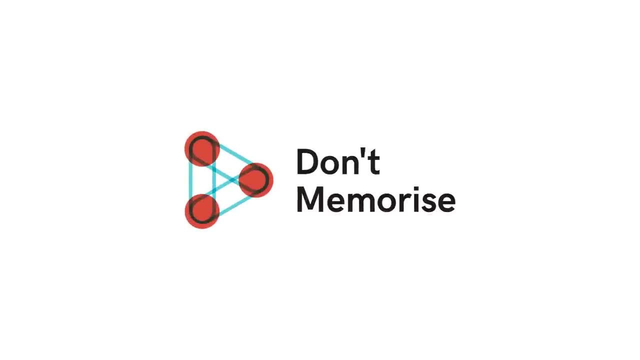 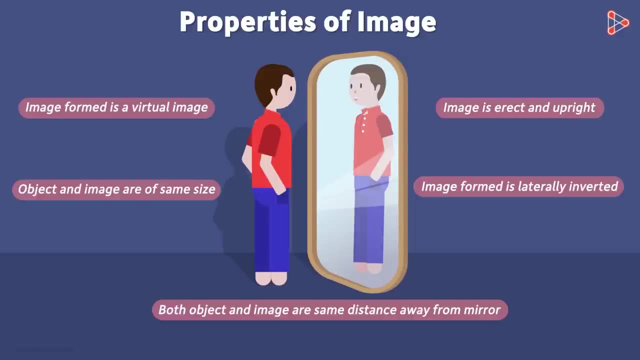 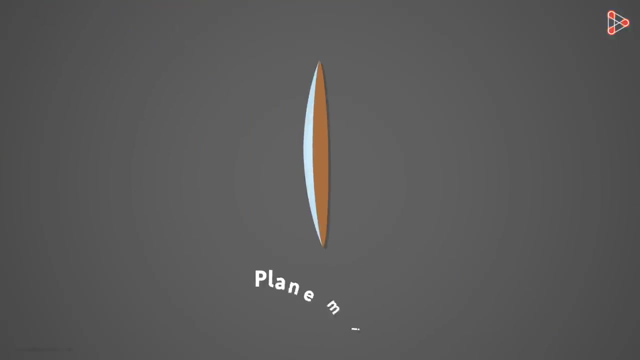 Till now, we have been looking at the properties of images formed by plane mirrors. A plane mirror is a mirror whose reflecting surface is flat. What about this mirror? Is this also a plane mirror? This is a mirror, as it has this smooth reflecting surface. 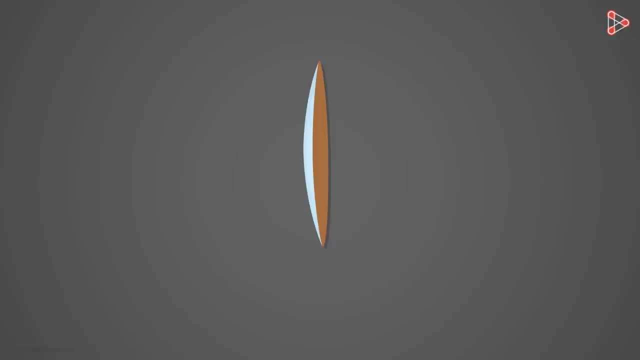 But this is not a plane mirror, as this reflecting surface is not flat. The reflecting surface is curved, and hence this mirror is called a curved mirror. What about this one? This is also a curved mirror. The difference between the two is that the reflecting surface of this mirror is curved. 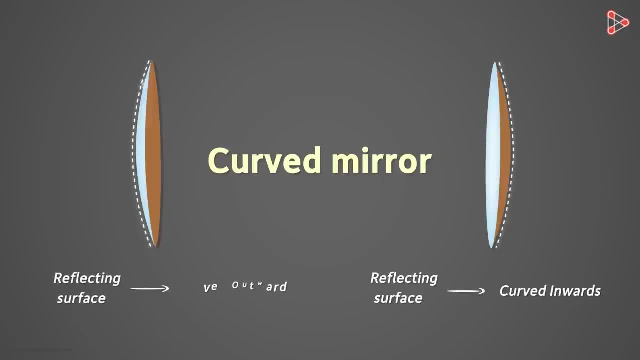 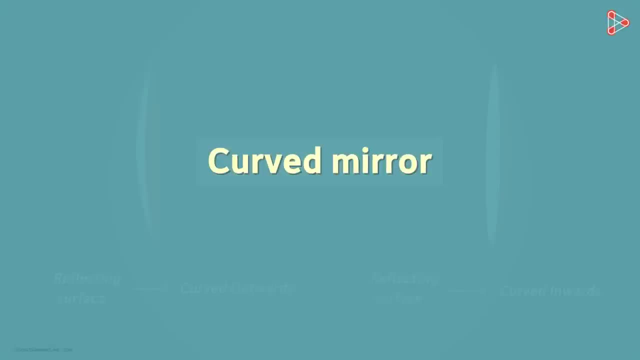 inwards, whereas the reflecting surface of this mirror is curved outwards. Can you think of examples where you have seen curved mirrors? A shiny surface of a spoon is a good approximation of curved mirror. It has two reflecting surfaces, One curved inside and the other curved outside. 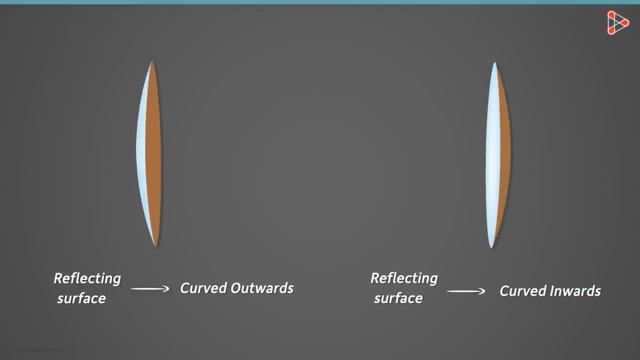 Now, the specific types of curved mirrors that we are interested in are called spherical mirrors. In fact, these two mirrors are spherical. Well, they look nothing like a sphere. But then why are they called so? They are called spherical mirrors because their reflecting surface is a part of a sphere. 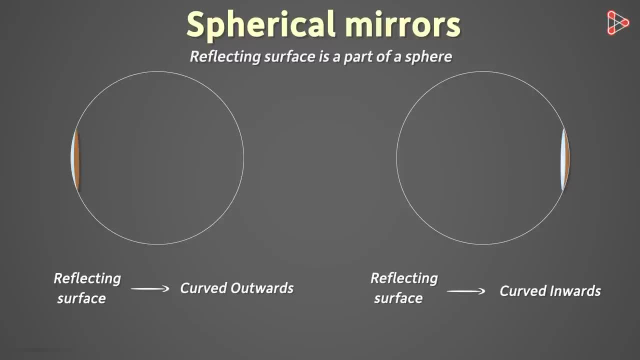 You can clearly see that the reflecting surfaces of both the mirrors form a sphere. The reflecting surfaces of both the mirrors form a sphere. The reflecting surfaces of both the mirrors form a sphere After. the reflection surfaces of both the mirrors form a sphere. Now, both these are given special names. 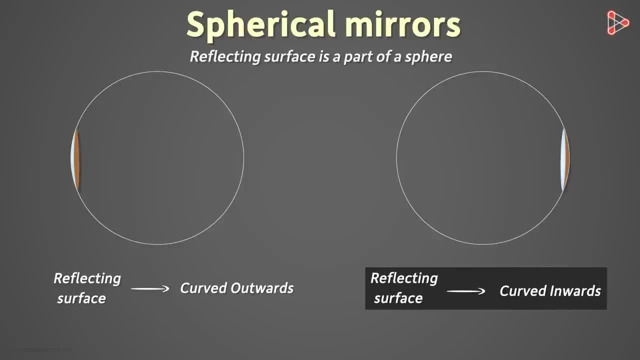 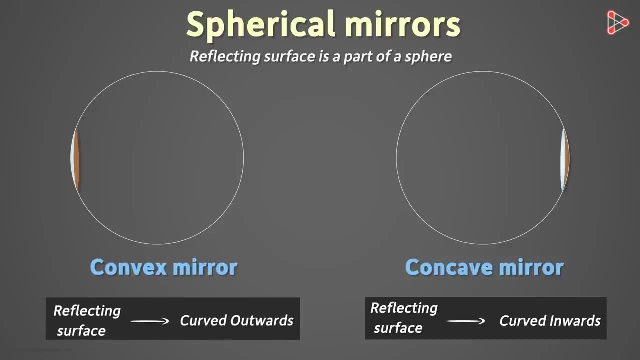 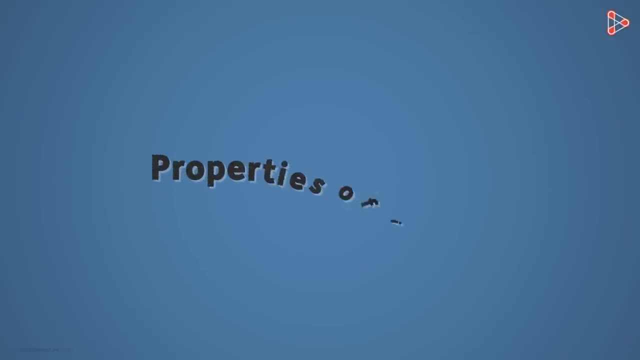 The mirror that has its reflecting surface curved inwards is called a concave mirror, and the mirror that has its reflecting surface curved outwards is called convex mirror. Yes, inwards and outwards. Now we want to study the properties of images formed by spherical mirrors. 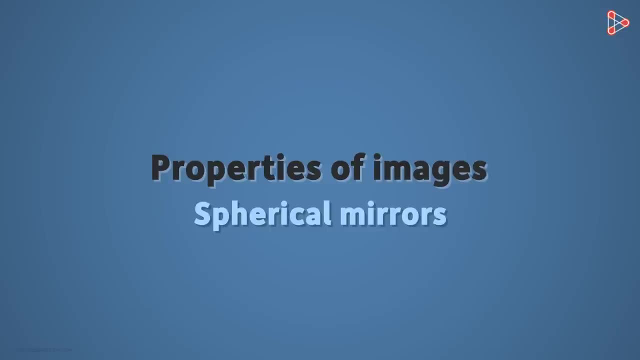 But before that, we need to define certain terms and expressions for these two types of mirrors, certain terms related to spherical mirrors. So let's do that. Both the mirrors are placed like this: Concave mirror on your left and convex mirror on your right. 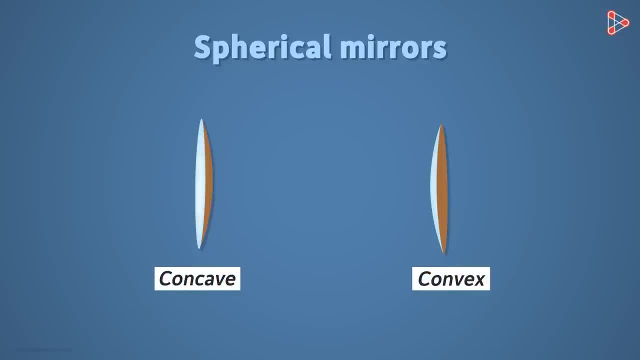 I am going to define the terms for both these mirrors: Concave inwards and convex outwards. The centre of the reflecting surface of the mirror is called the pole. We represent it with a point P In the front view of both the mirrors: you.